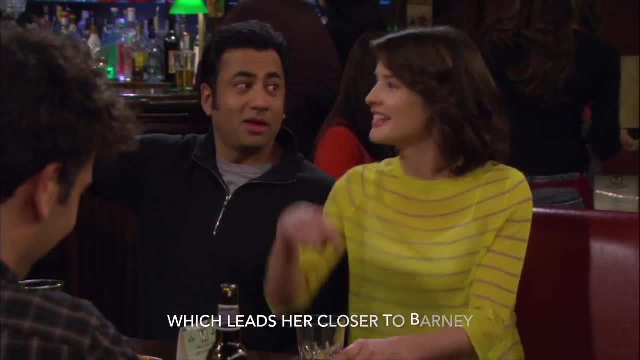 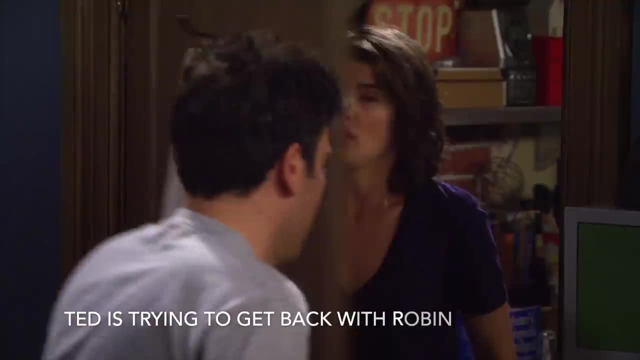 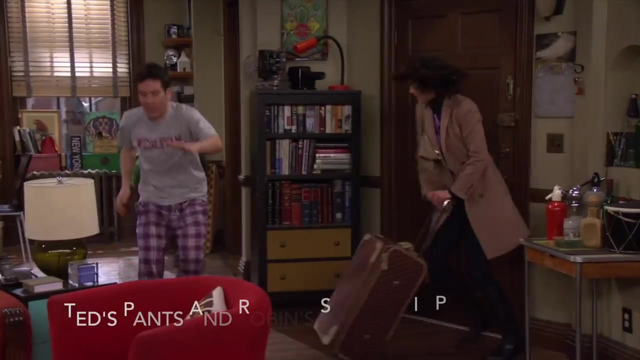 Whoa, It was small, but I think I felt something Top 10 things Lily said on her wedding night: Ha ha, Stop laughing at it, Lily. I go camping in secret. You're back down. Where are my shoes? 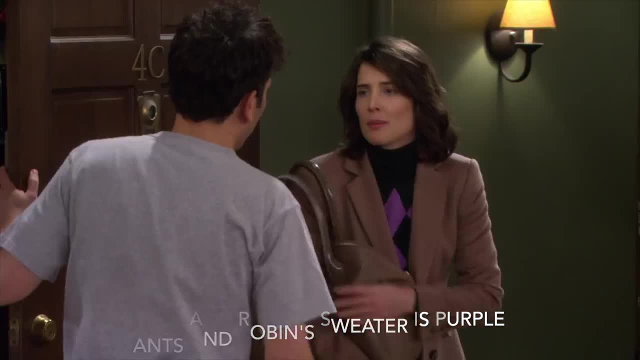 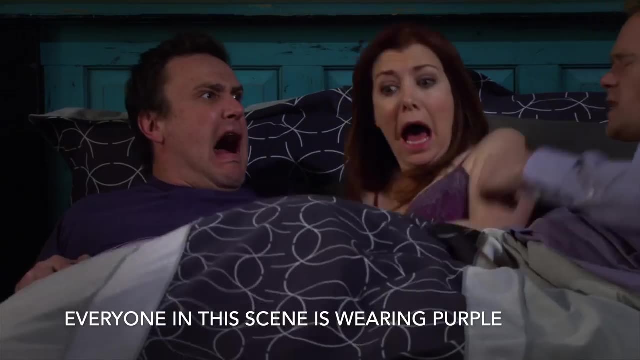 Where are my shoes? Don't worry, It's fine I can look about all this. Yeah, just go Goodbye. An AF Man, Tim, really needs to work on his boundaries. Shh Guys, seriously, Why are you in our bed? 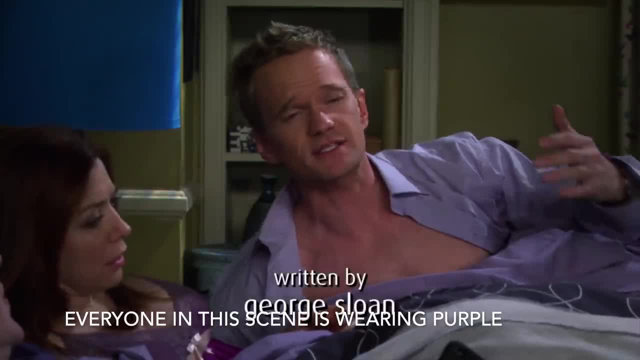 I took the drunk train and got stuck out here. Oh God, I am so hungover. Oh God, Lily's, It's not gonna happen, is it? Sorry? Do you love me? I love you, I love you. 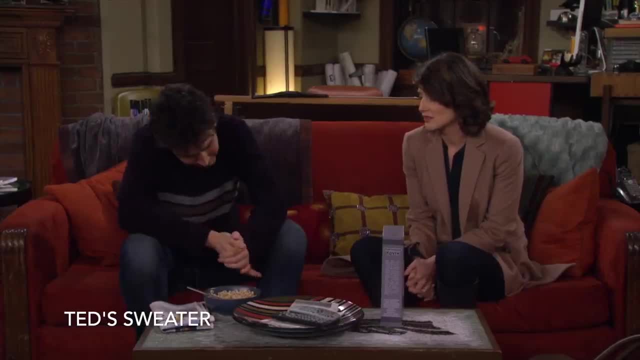 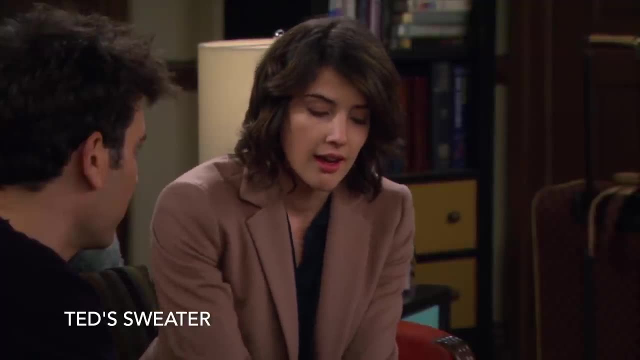 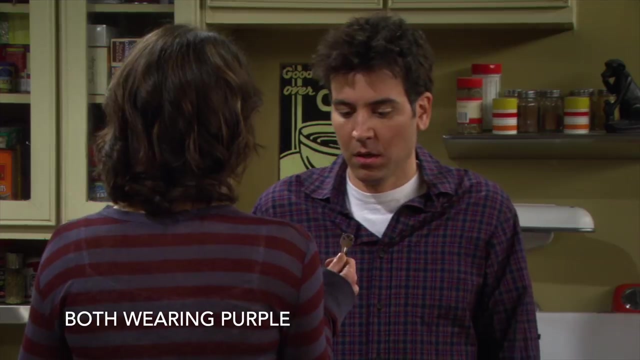 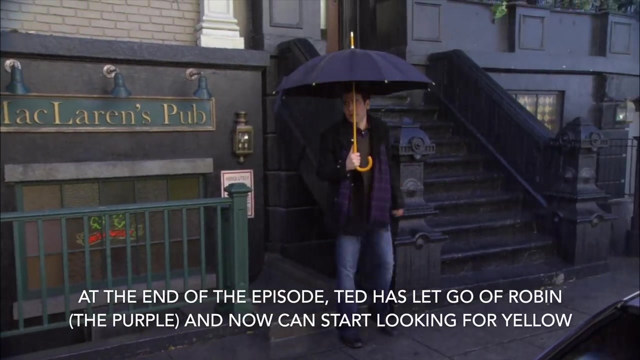 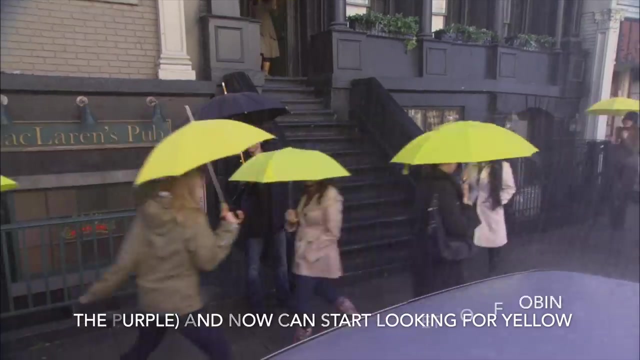 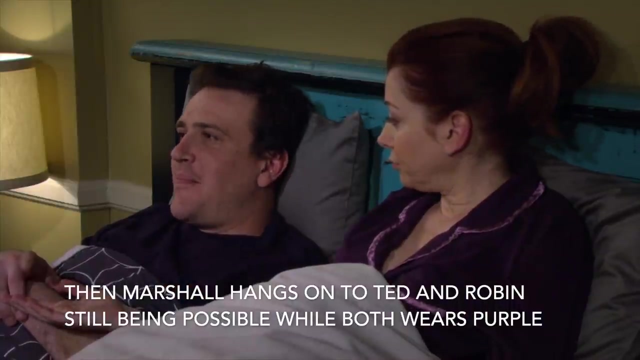 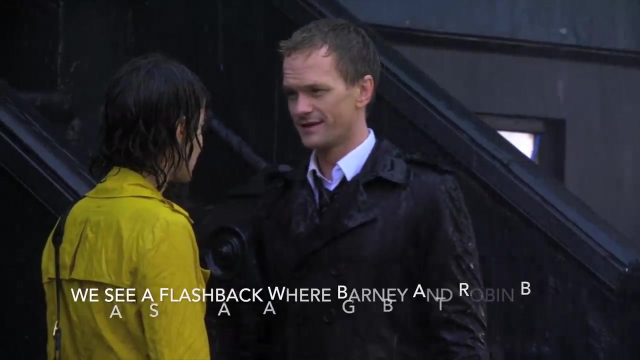 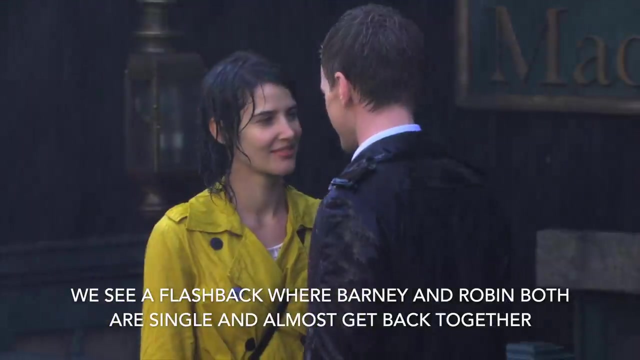 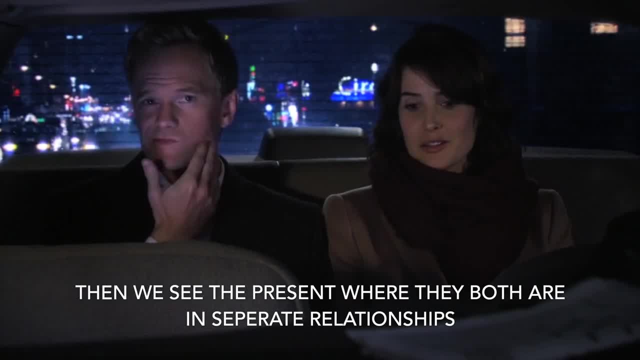 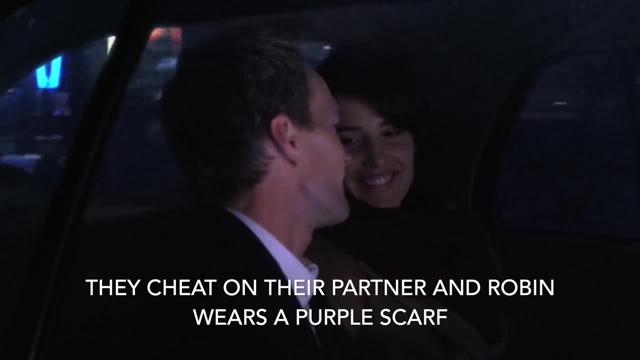 Good thing we didn't. Yeah, I mean, not long after that you got together with Nora. You met Kevin. Disaster averted Exactly. I would have ruined everything. I would have been all I know right. So dumb. 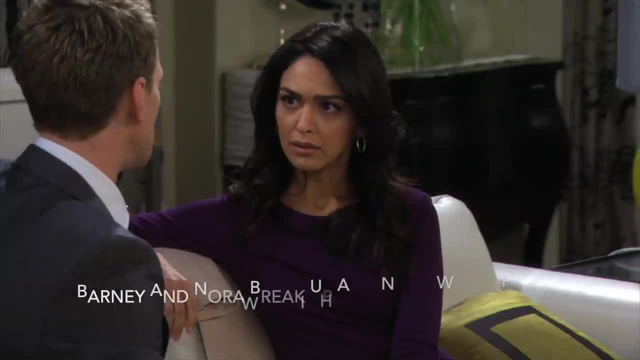 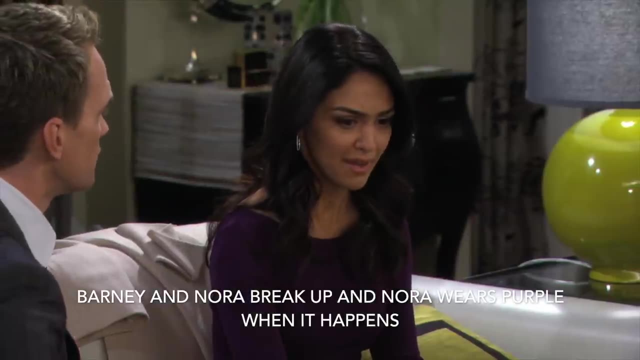 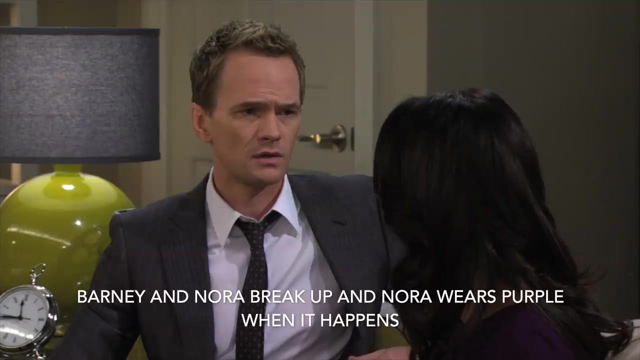 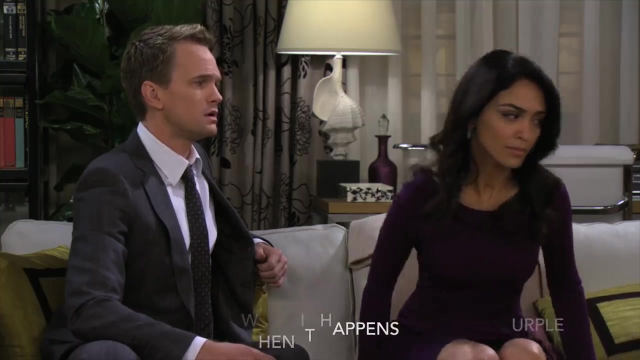 I cheated on you. I don't even know how to react. I am so sorry. Is this a one-time thing? Can you tell me it didn't mean anything? No, Wow, You have enormous penis syndrome. I've never heard of that. 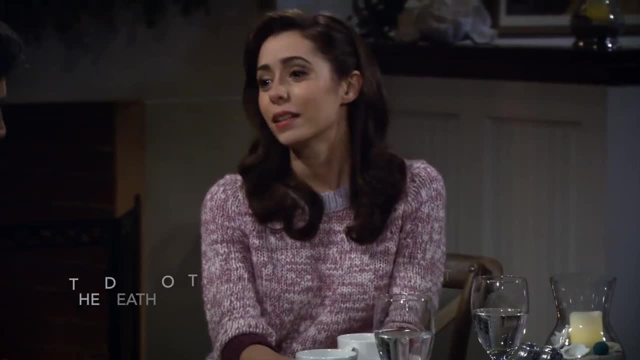 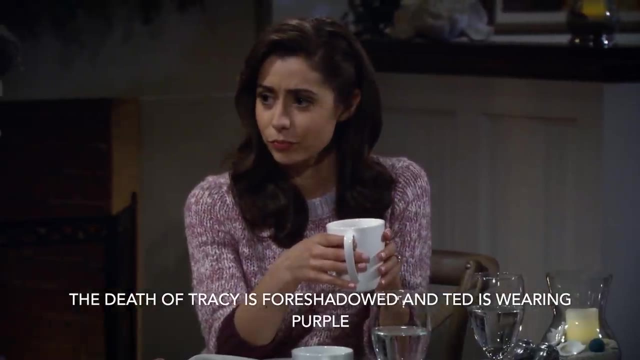 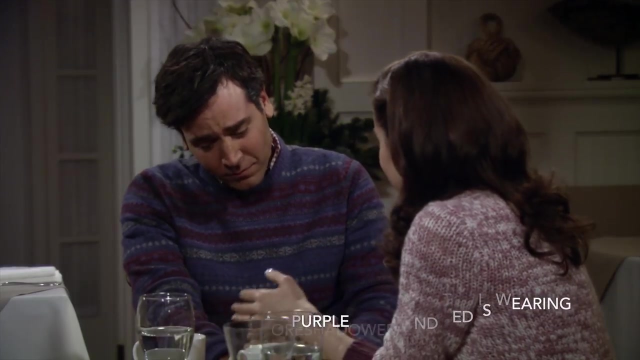 Yeah, that's the problem with EPS: Lack of awareness. Yeah, of course she showed up. What mother is gonna miss her daughter's wedding? Oh, hey, No, Come on, It's okay, I'm a full girl on that train platform. 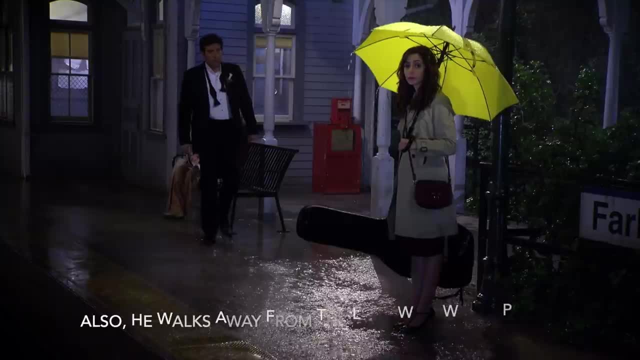 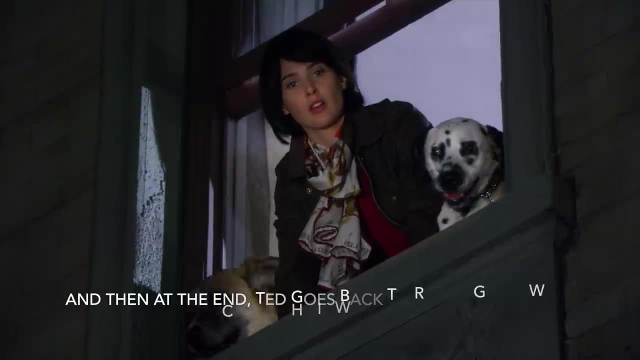 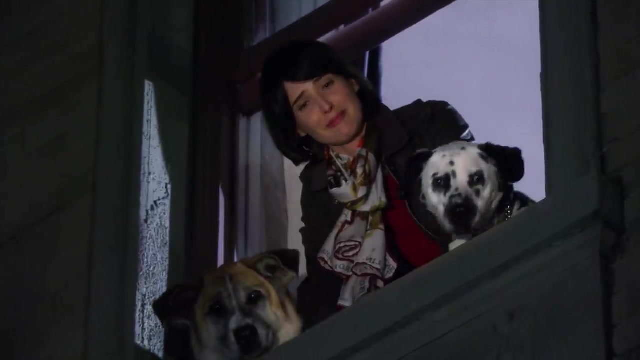 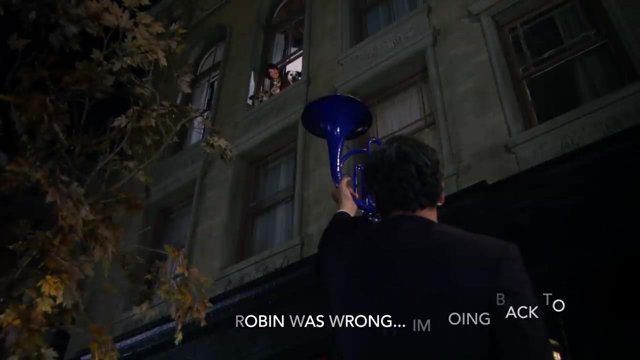 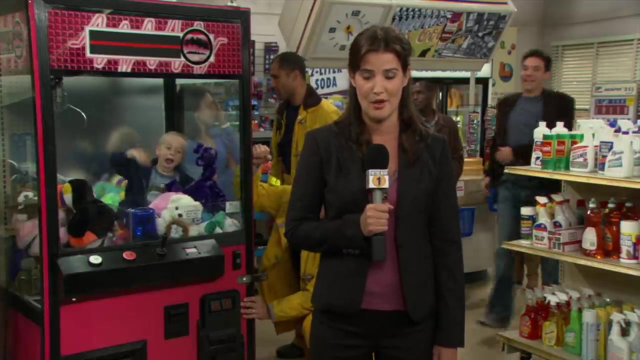 And that I had the guts to stand up, walk over to her, tap her on the shoulder, open my mouth and speak, All in the pursuit of a stuffed purple giraffe From Metro News 1,. I'm Robin Shabatsky. 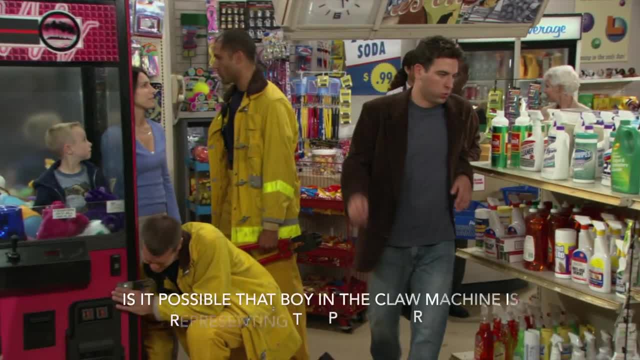 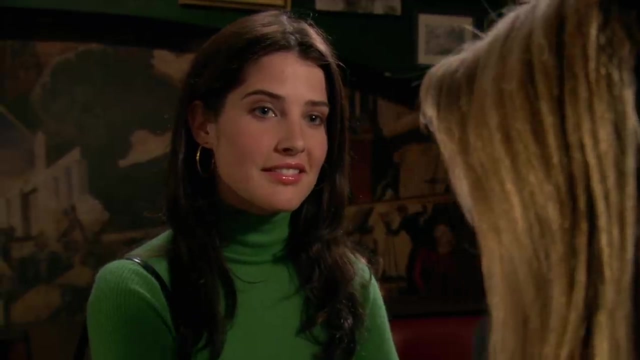 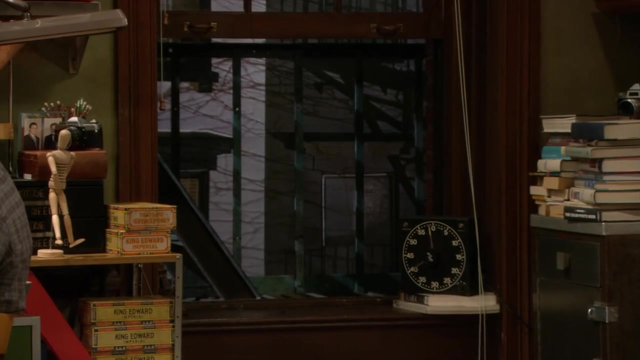 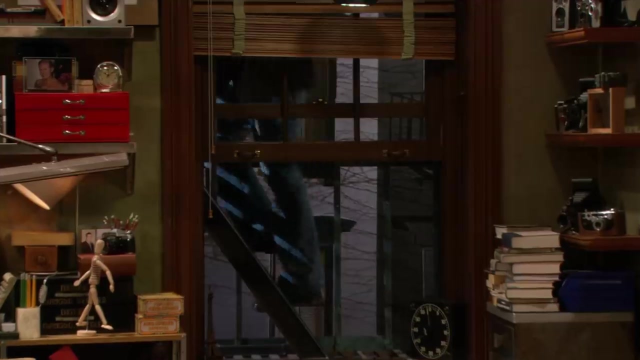 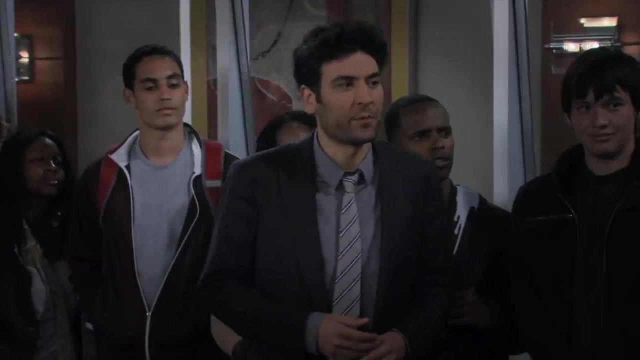 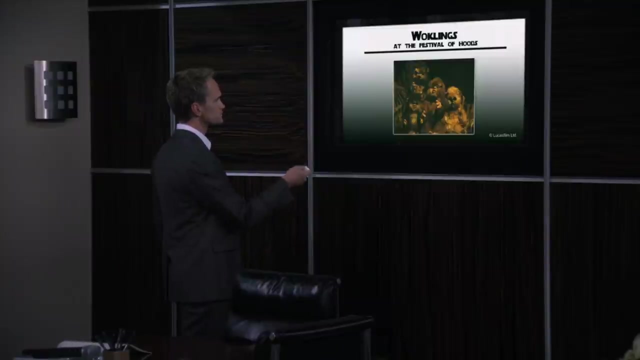 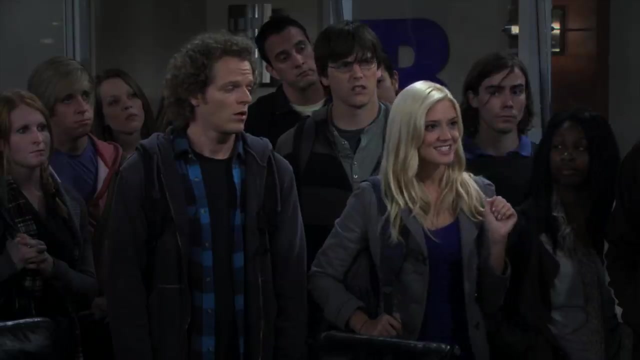 We're clear. Thanks, Don. How was it- I have a rich backstory- that the movie didn't really go into? Barney, why don't you just skip to the part, Fine? ah yes, ultimately, they reminded you of our teddies. they reminded you. 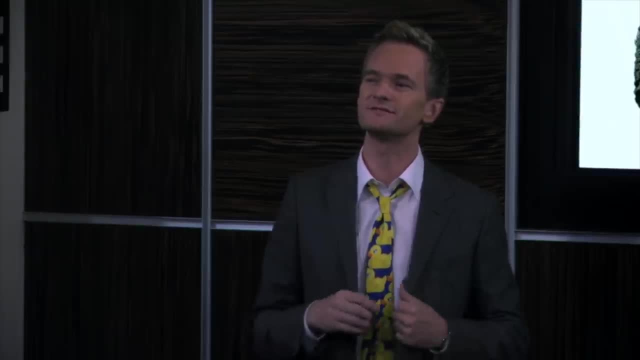 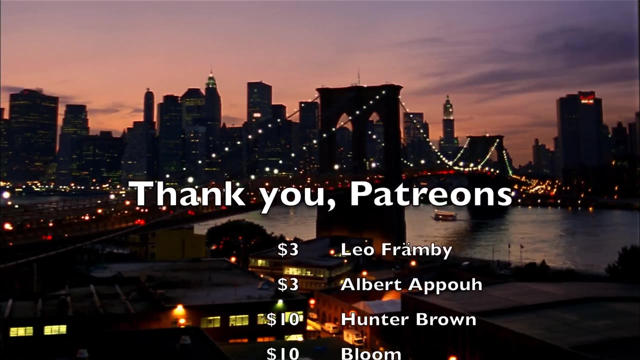 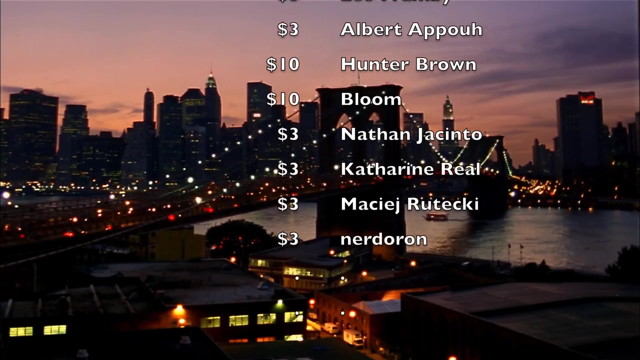 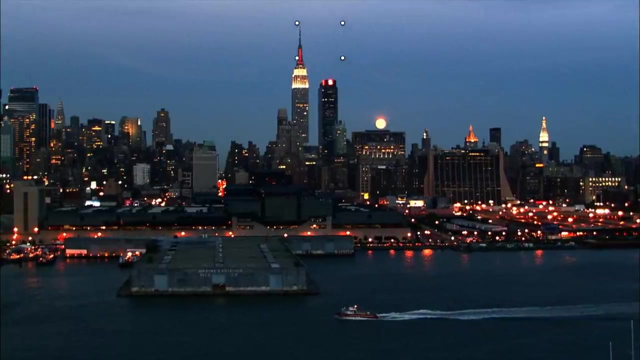 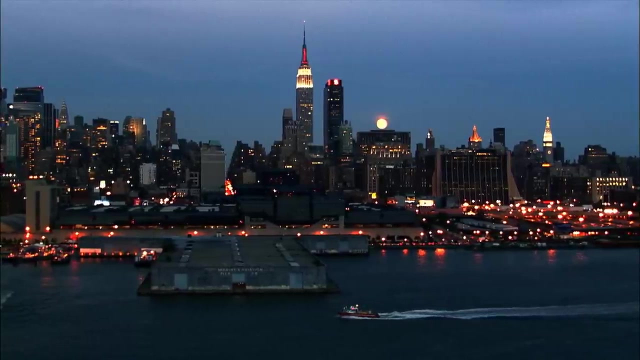 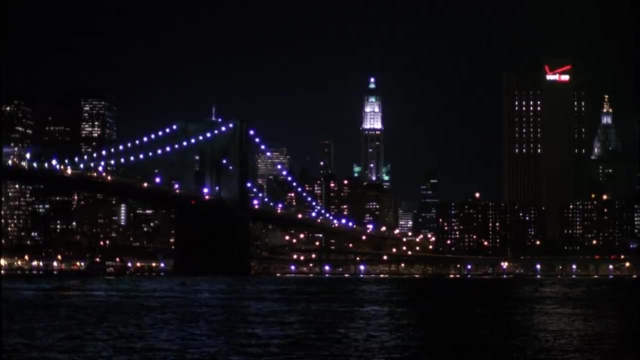 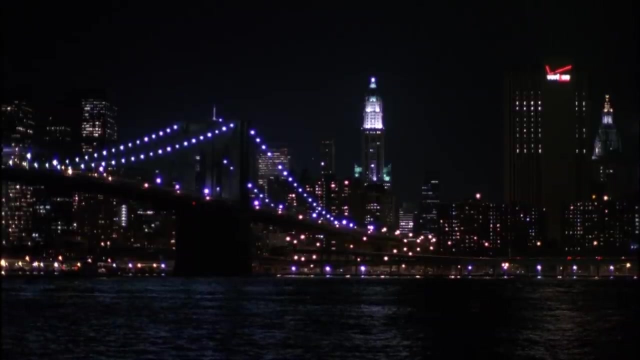 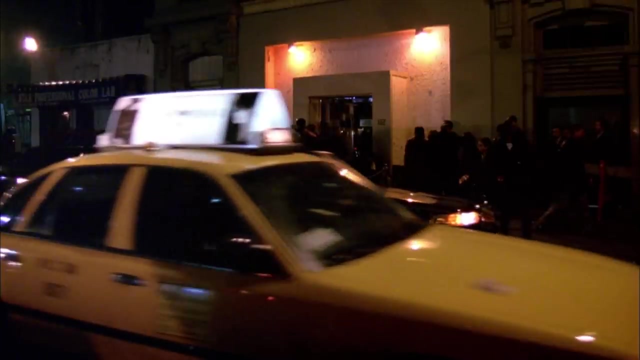 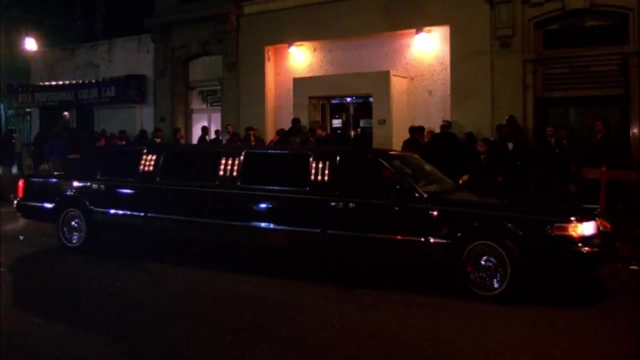 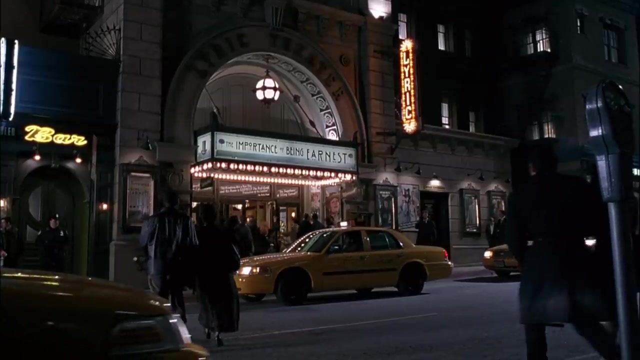 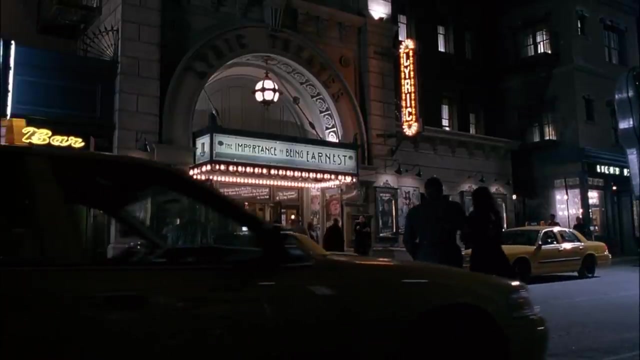 of your teddies. thank you, gina. how do you know her name you? Thank you, Thank you.